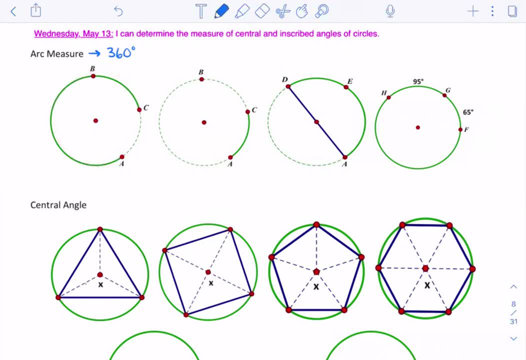 That's a big arc, Mrs Tahami. Yep, That's a large one, And if I go back to my notes from Monday, I realize that that is more than half the circle that is colored in green and that's called a major arc, Exactly Now, if I don't exactly use the word. 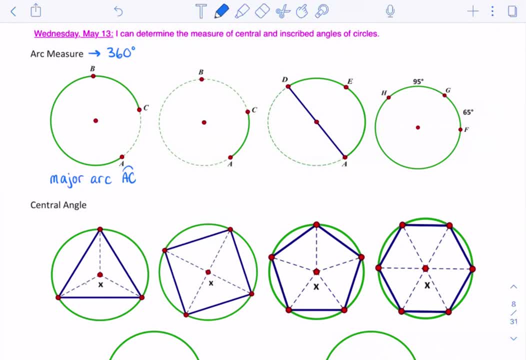 major arc. if I just want to tell you, Ms Murphy, find me the measure of arc AC, but I want you to find the major one. I would just say arc ABC And that should be enough, because that tells you you have to go from A and you have to touch B next, You cannot pass through C. 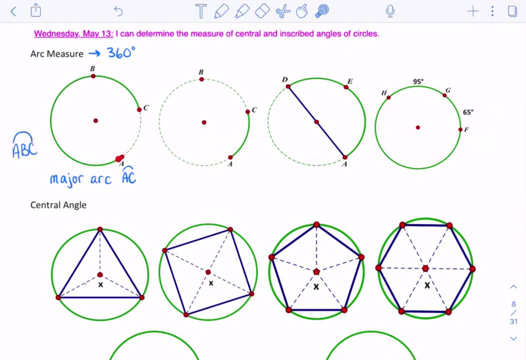 So if I say arc ABC, I'm going to go from A to B. next, You cannot pass through C. So if I say arc ABC, it means I have to go the bigger way and go from A to B to C. So if I just say arc AC. 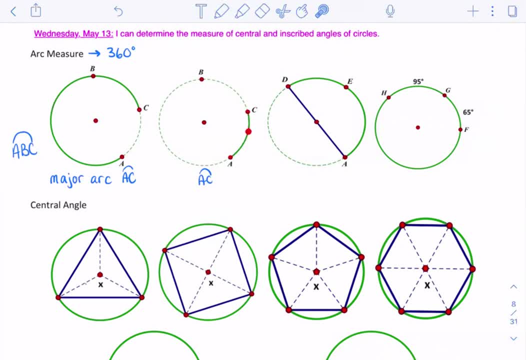 you can always just go the fastest route from A to C. So if I did not want to use the words major or minor arcs, let's say I cross this out. If I wanted you to go the major way, I would have to say ABC. If I wanted you to go the minor way, 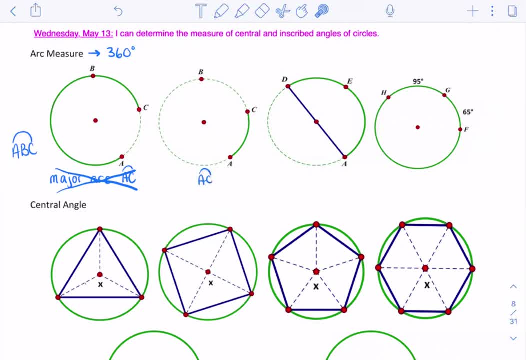 then you would just say AC. Okay, that's clear, Great. And then do you remember if I have a diameter, how many degrees this arc is? That is a semicircle, it's a hemisphere. So half of 360 is 180.. 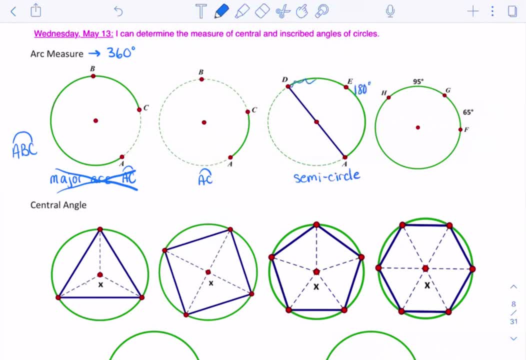 So that means this arc is 180 degrees, this whole entire arc. So if here I have arc HG And GF is 65.. What is the measure of major arc HF? So I have to take 360 and subtract what I know I have. 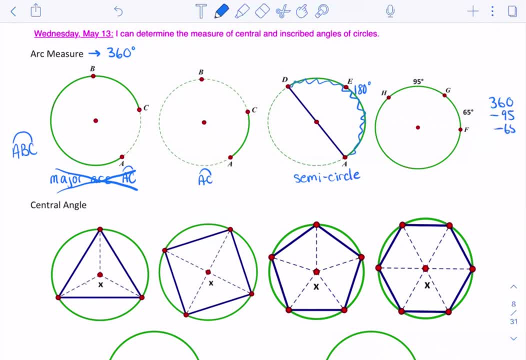 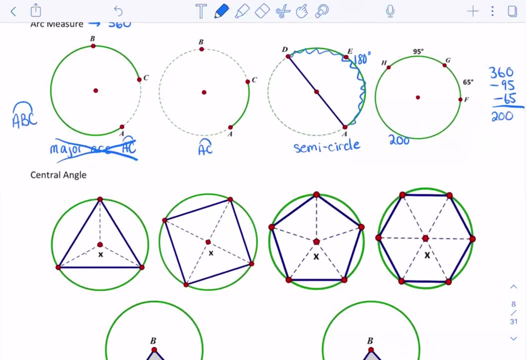 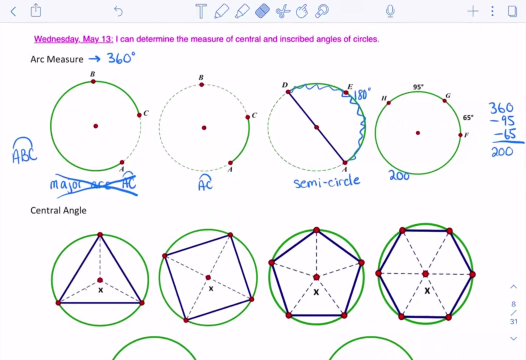 So 360 minus 95 minus 65 is 200.. Very nice work. So on that one, Mrs Talhami, I would have to say just HF, Because if I said HGF that would actually be the minor arc that time. 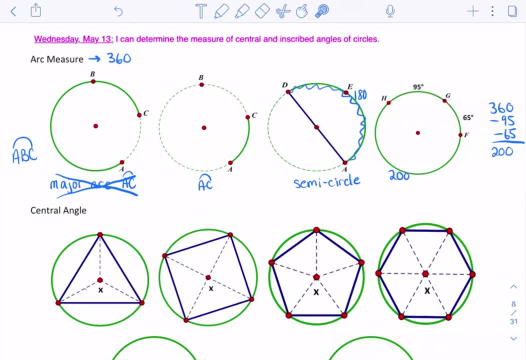 Right. If you said HGF, it would give me the minor arc. That's why I said major arc, HF, Because there is no point here for me to specify. I want you to go the major way, So I do have to use the words major arc. 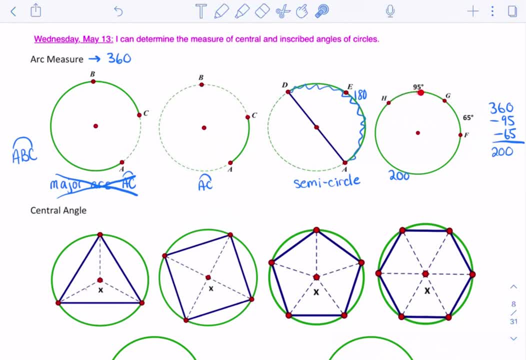 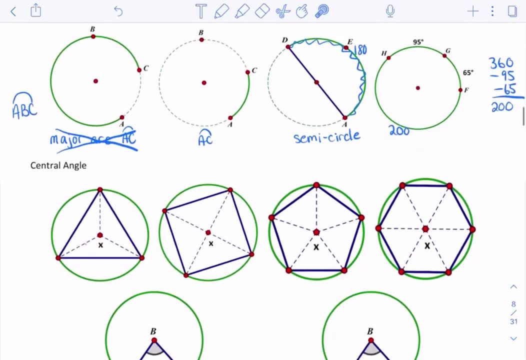 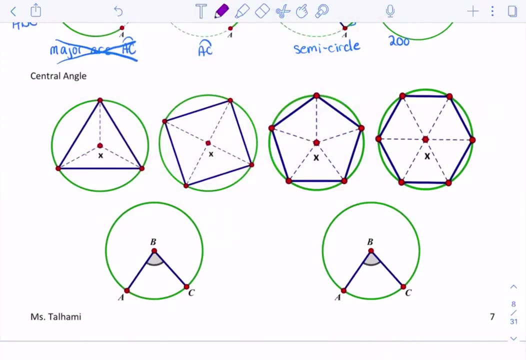 Because if I don't- and I just say HF- it's assumed that you could go the minor way. All right, So let's talk about this first word that we mentioned in our goal today: Central angle. What do you hear in the word central? 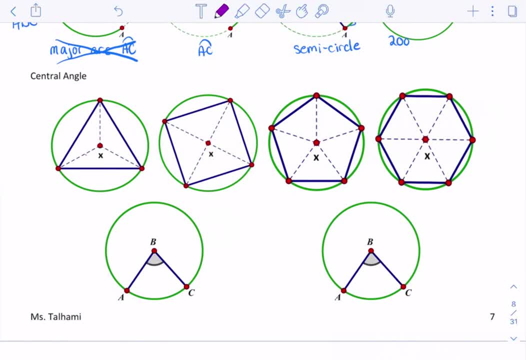 When I see the word central, I think of center. Good, So a central angle is an angle whose vertex is on the center of the circle. So here is an example of a central angle. This would be a good place to pause the video so you can write it. 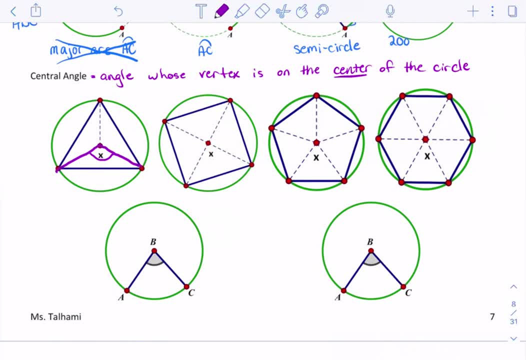 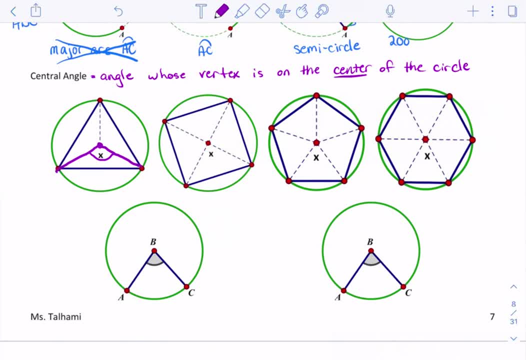 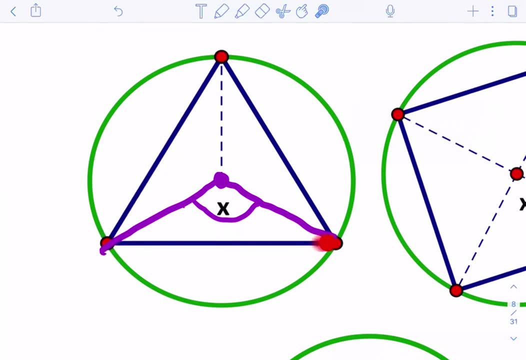 Absolutely So. if we take a look at this, this picture right here- we're not going to go through all of them, but let's just focus here. So, Ms Murphy, let's just say this was an equilateral triangle where all three sides are equal. 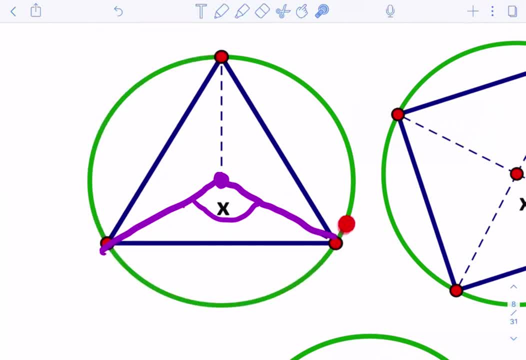 What do you think is true about all three of these arcs? then They must also be equal. So if they're all equal, how many degrees is each arc? Well, I know, all together it's 360 degrees. divided by three equal parts would give me 120 for each of those angles. 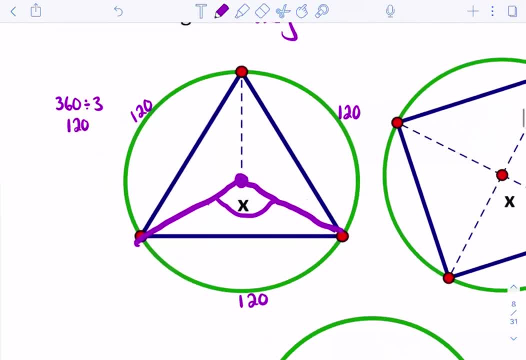 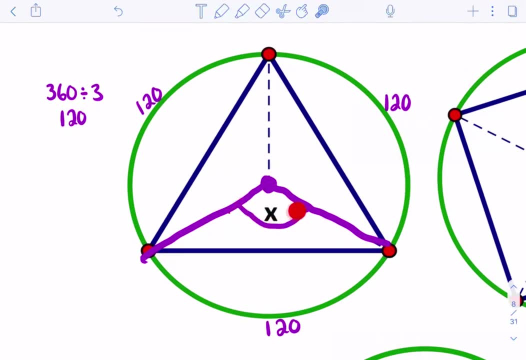 You mean arcs, Not angles, arcs, Arcs, Right? Great. So that's, that's wonderful, And I love the math that you did there. So let's also take a look here. Right, We have one, two. 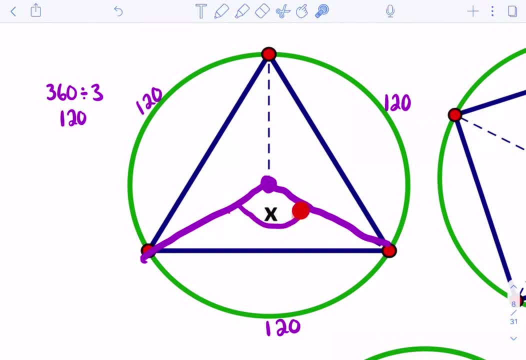 three central angles that make up the whole circle. So how many degrees do you think each one of these angles is? Those would also be three equal angles, So each one would also be 120 degrees. Oh, so hold on, Wait a minute here. 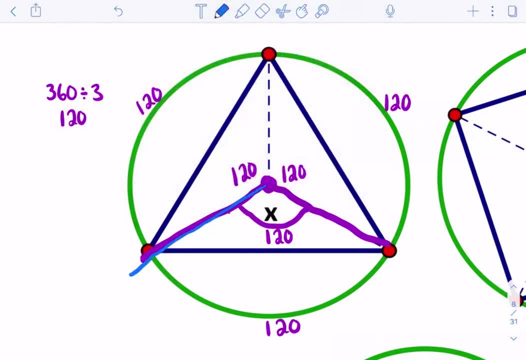 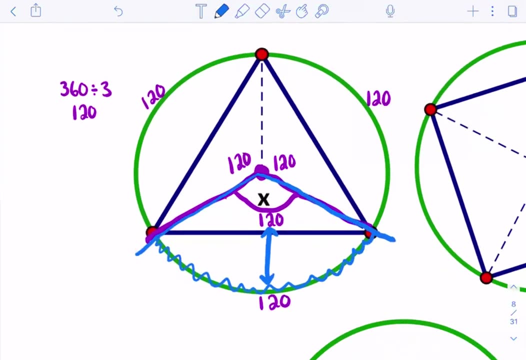 If I have a central angle that cuts the circle- and we'll use a different word in just a second- Does that mean the arc is equal to the angle? Looks to me like it is Good, So I'm going to actually call this part of this. 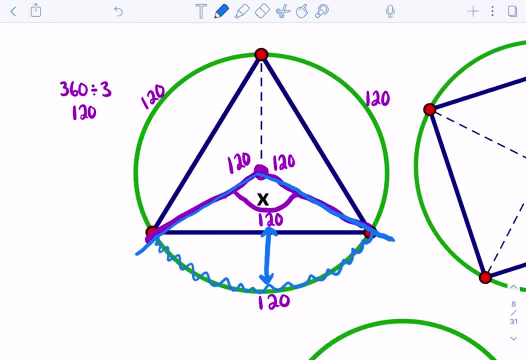 this section of the circle here that it cut the intercepted arc. Intercepted because you drew a line right through it from the vertical. It's like a vertex on both sides. You're intercepting, It's like it's like intercepting. 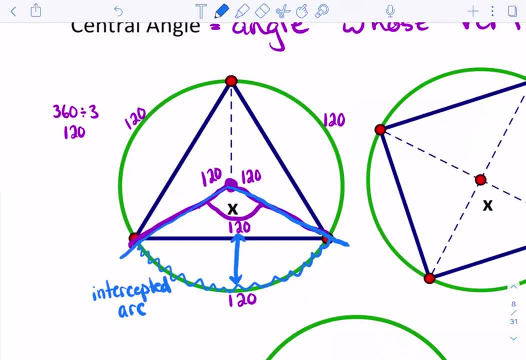 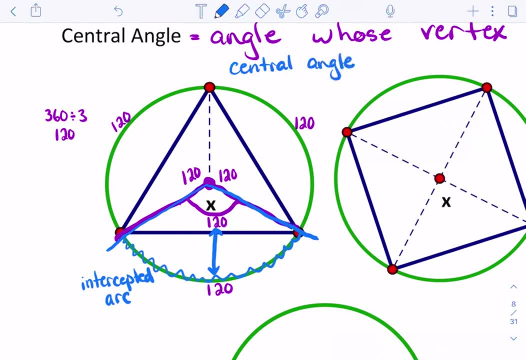 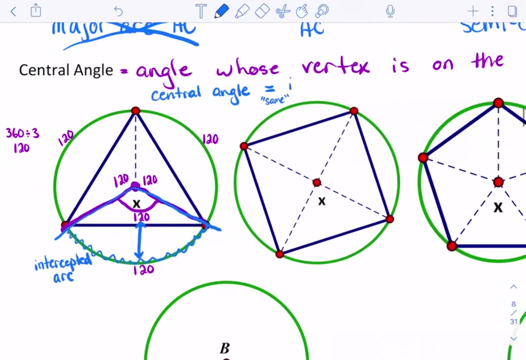 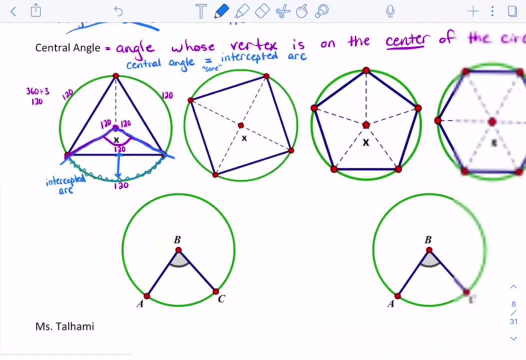 but it's called intercepted arc, So I'm going to write that as a rule here. So the central angle is the same or equal to. we could say central is the same as its intercepted arc. So that's what I want you to learn about. 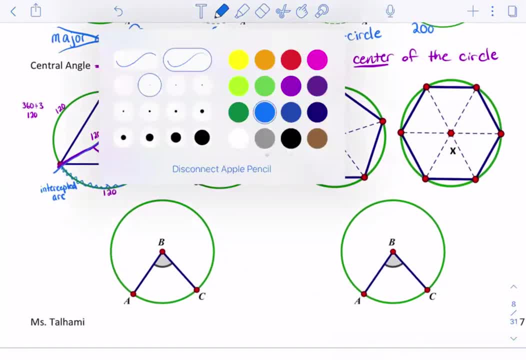 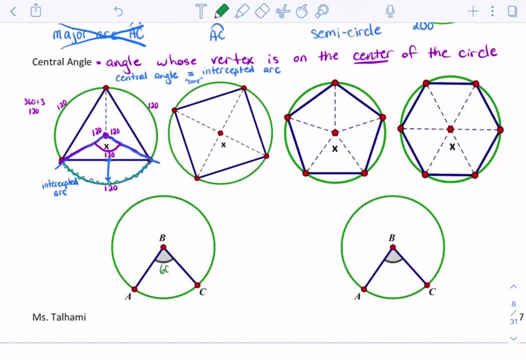 It's central angle. So I'm going to give you two quick examples here, If you look. so let's just say, in this picture this angle is 60 degrees And in this picture the arc is 80 degrees. Do you think? let's say, Miss Murphy? 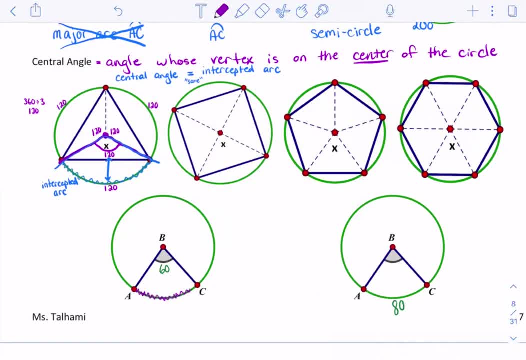 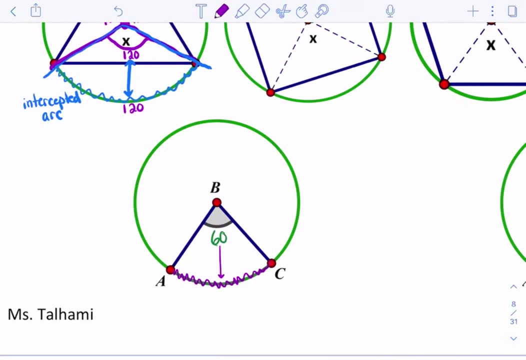 do you think you could tell us the degrees in this arc AC? Yes, it's the same as the angle inside 60, because it's coming from the center. So the central angle is the same as its intercepted arc. Cool, So then what about in this one? 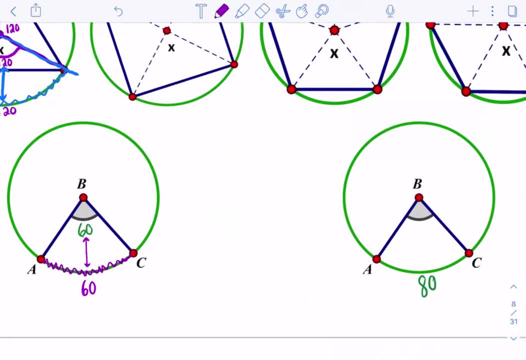 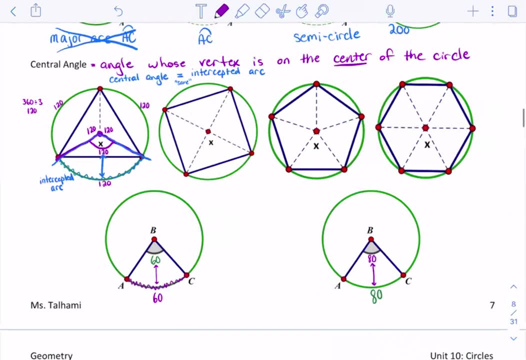 What is the measure of angle? B Must also be 80. They equal each other. Wow, Okay. So then in the, that is what you need to know about a central angle. If you want to pause it here, please pause it and make sure you know. 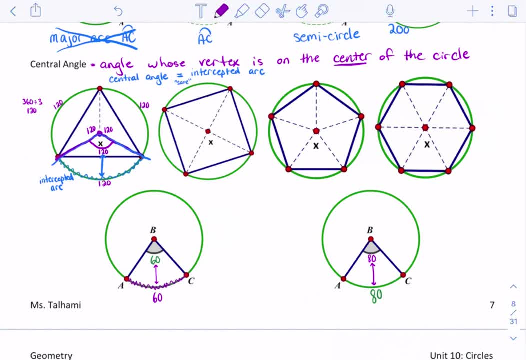 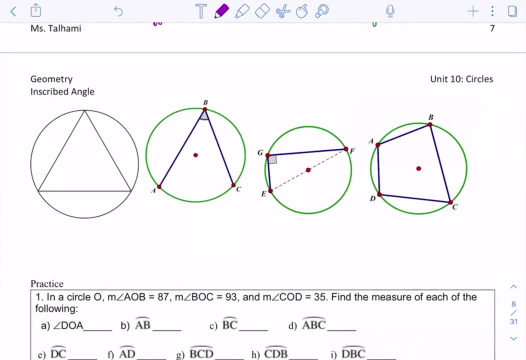 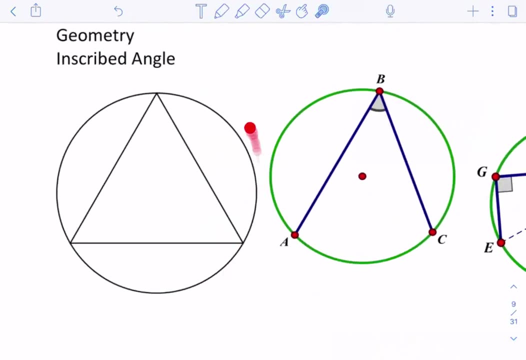 Make sure you get down what you need, because that's what you need to know about a central angle. And the second kind of angle I want to discuss with you is called an inscribed angle. We actually have heard this word inscribed before and actually looks just like this picture. 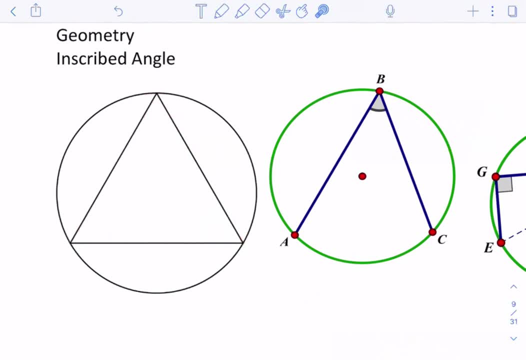 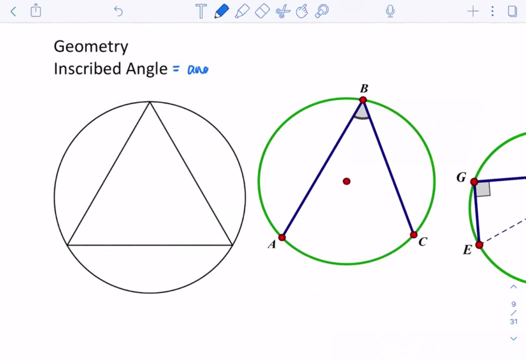 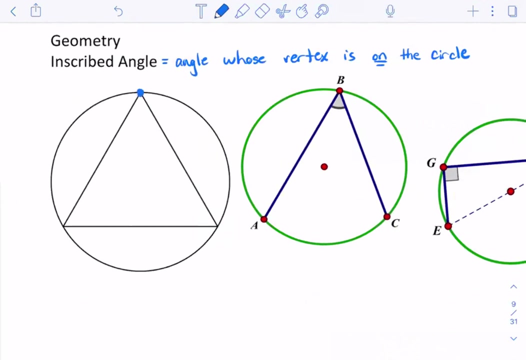 This triangle is inscribed to the circle because it's inside and its vertices are on the circle. And that's exactly what an inscribed angle is. It's an angle whose vertex is on the circle, So, instead of the vertex being in the center, it's actually touching the outside of the circle. 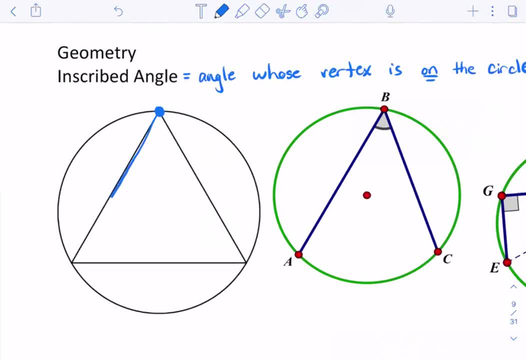 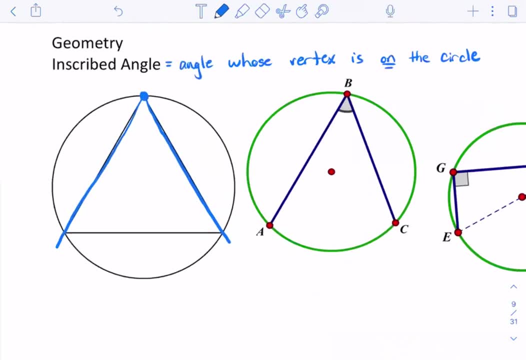 So here's oops. You're right, Mrs Talhami. We did learn about inscribed. I remember when we did constructions We had to construct An equilateral triangle. Yes, we did, Yes, we did. 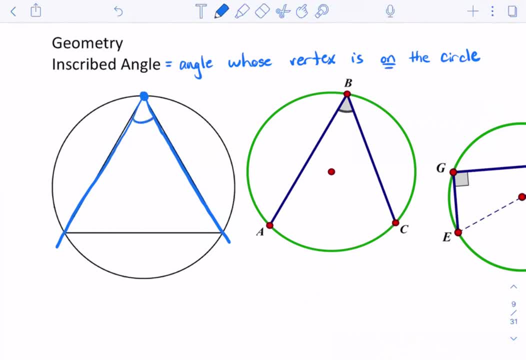 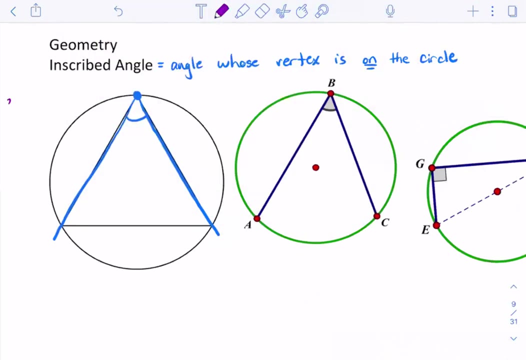 So if you look at this angle right here Now, I want us to go back to that thought, Miss Murphy. We said: if this was an equilateral triangle, how much was each one of these arcs? Well, an equilateral triangle has three equal angles, and all triangles add up to 180. 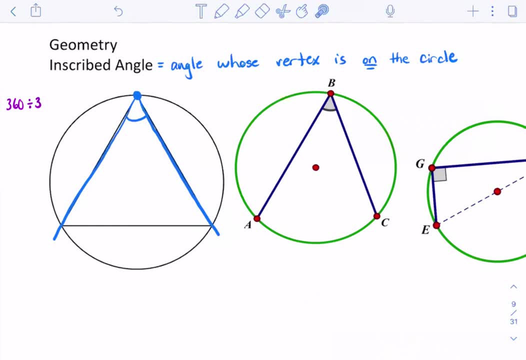 So each You're going from a different point of view, I think, than I am right now. Yep, I was each one of these arcs, So that means that each one of those arcs are also equal, So each one is 120.. 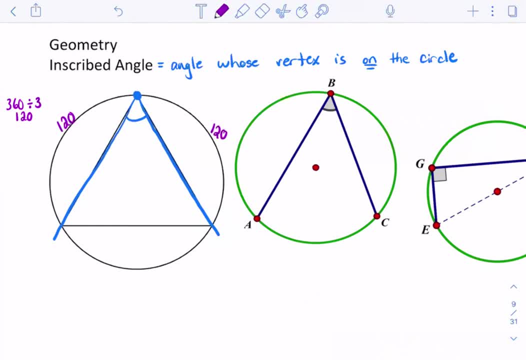 Good, So that's what we said earlier And then I think the thought that you were just having Miss Murphy is we were. you were talking about the angles inside the triangle. Yes, So the angles inside the triangle have to add up to how much? 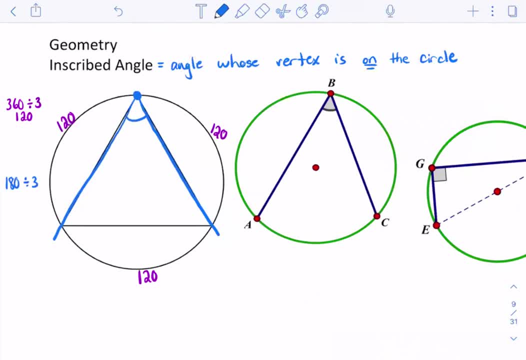 180.. Divided by three, because they're all the same- is 60.. So each one of these angles inside the triangle is 60.. So what is the relationship between an inscribed angle and its intercepted arc? Well, I know, if I double a six, I get a 12.. 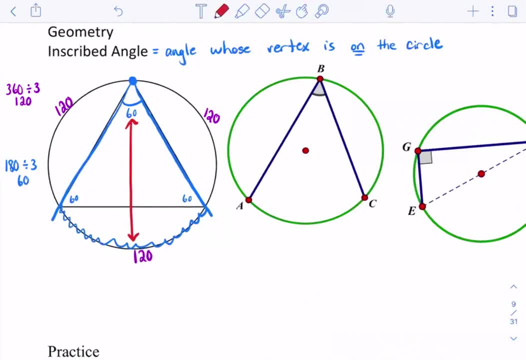 60 doubled is 120. So it looks to me like you are doubling When you have an inscribed angle. So the intercepted arc is two times the inscribed angle. Or let's write the other way: The inscribed angle, If we go backwards, that must mean it's half. 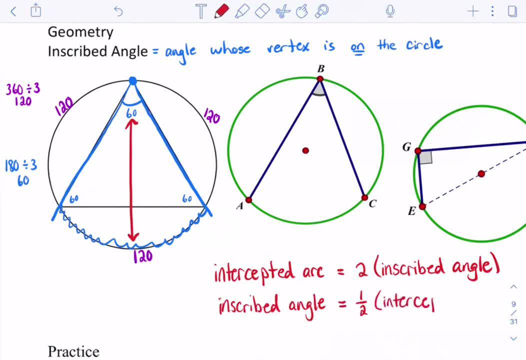 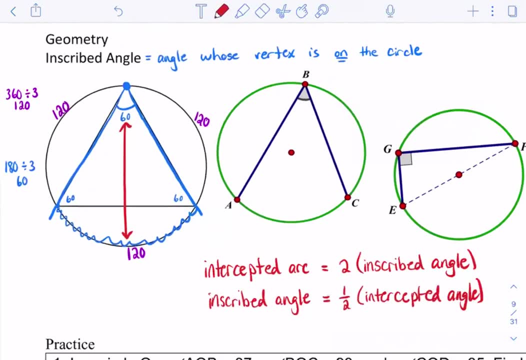 It's half of the intercepted arc, So So So. So if you need to copy this down, you can, Or just remember. it's a double half rule where the arc will always be double And the inscribed angle will always be half. 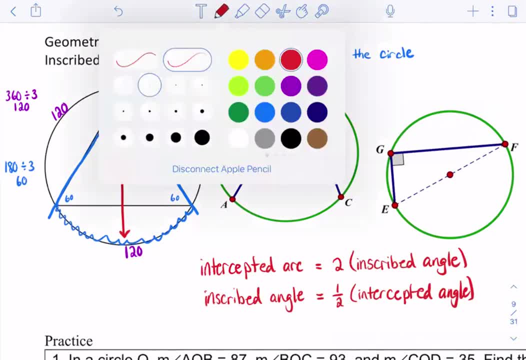 So it's a double half rule. So in this example It kind of looks like that. Mrs Tahami, That shouldn't be too hard to remember, because it looks twice the size that arc and the inscribed angle It does. 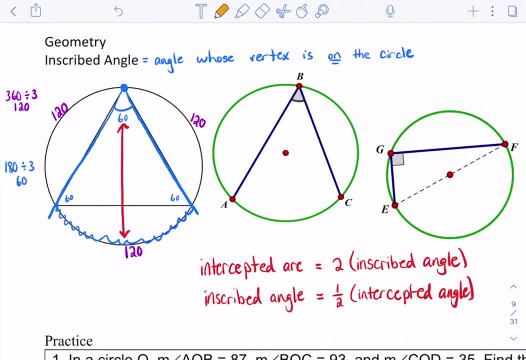 So if we take a look here in this example, let's just say this was 140 degrees in this arc AC. What does that mean? angle B is Must mean that it's half of 140, which makes it 70.. Very good. 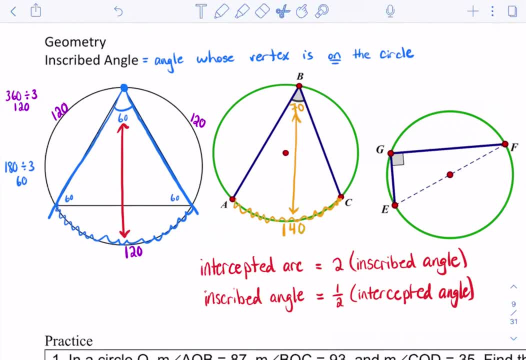 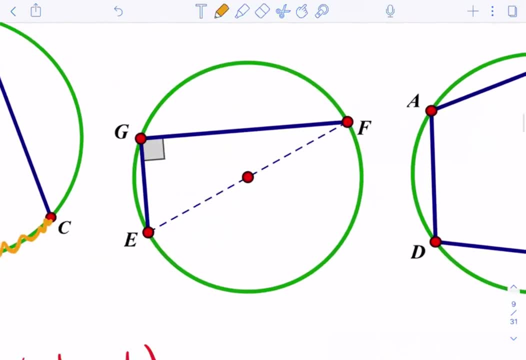 The intercepted arc is twice the inscribed angle, Very good. And then- this is actually very important- It's important to recognize: Do you see what this angle intercepts? I always like to trace my pen or pencil to really see what it intercepts, what part of the circle it cuts. 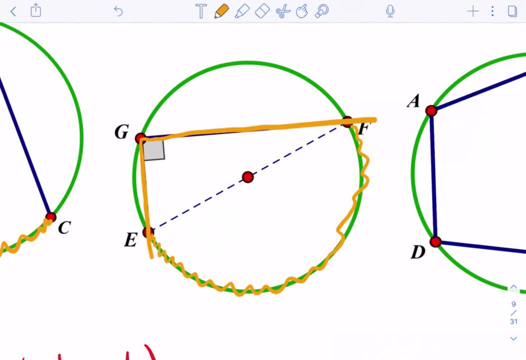 How much of the circle does it cut here? Half the circle, Half of the circle is 180 degrees. So that means the inscribed angle here is how much? 90. And that's exactly what it's marked off. So that's really important to recognize because once you have a right triangle, 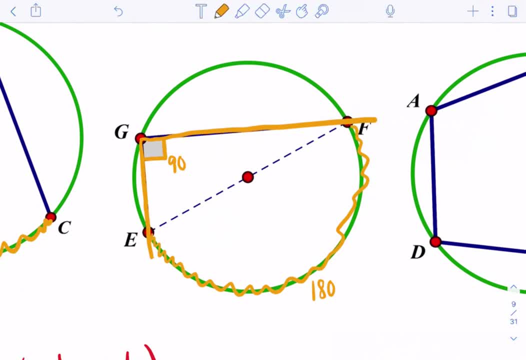 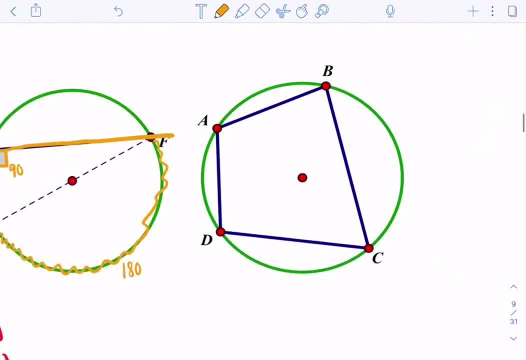 a whole bunch of information that we learned about right triangles can now be applied here if I needed to, And then this last piece, So this is a really cool thought. Let's kind of put this all together, So I have an inscribed quadrilateral. 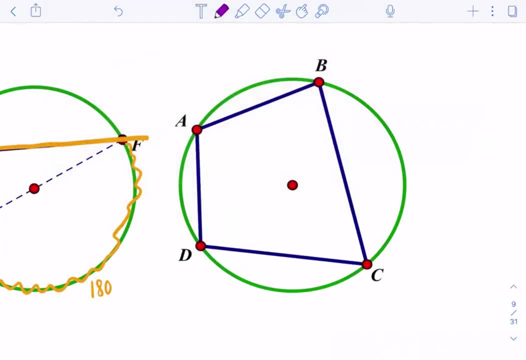 Now notice that it's not called a parallelogram, It's just a quadrilateral shaped with four sides, And I want to know: Is there any type of pattern or rule that might happen here? So I'm going to ask Miss Murphy something. 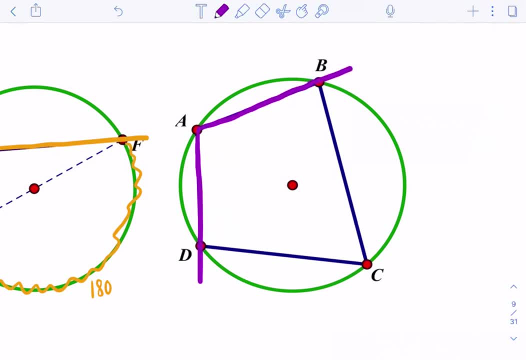 Let's just say that angle DAB is 100 degrees, Miss Murphy, What do you then know? Well, I see that that's touching the circle. So that must mean that DCB, That major arc, must be double, that DCB must be 200.. 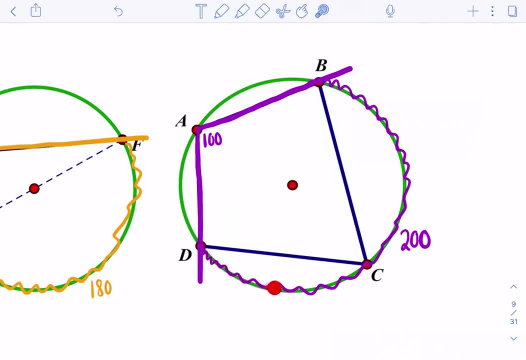 Great. And if you know that arc DCB is 200, what do you know? that the arc DAB, which is the rest of the circle, how many degrees would be in that? Well, a full circle is 360, minus the 200 that I already have would leave me with 160 degrees. 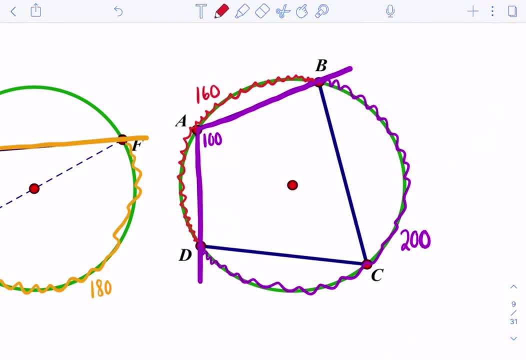 So if that's 160, what angle is inscribed to that arc? Inside would be over at angle C, and that must be half of 160. Which is, Which is 80.. Oh, so look what happened here. What do you see about these opposite angles? 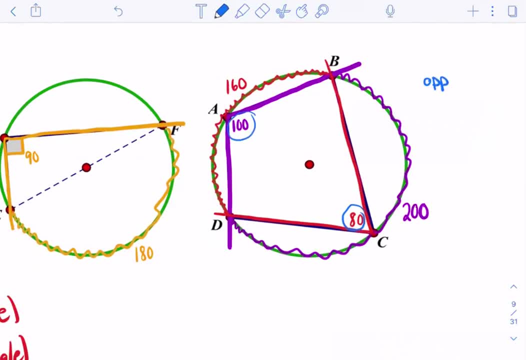 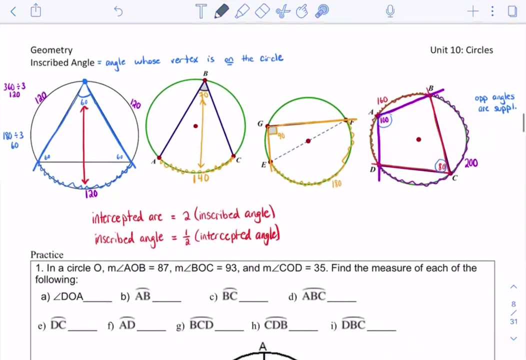 Ooh, they add up to 180.. Opposite angles are supplementary. Oh, that's very cool. Well, that's really what we want you guys to know about an inscribed angle. is this rule right here? So if you need to pause it and take down some notes, that would be great. 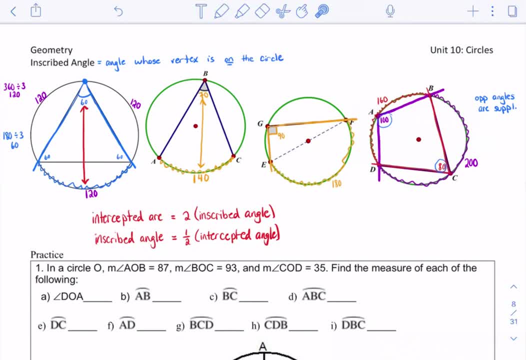 Miss Murphy, I know you said you had a meeting. I do. I still have five minutes, Okay. So, as the meeting starts, I think it's really helpful to do what you're doing. Mrs Telhami, I like that you're using colors and you're extending your lines through the circle so you can really see which parts of the circle we're talking about, what arcs. 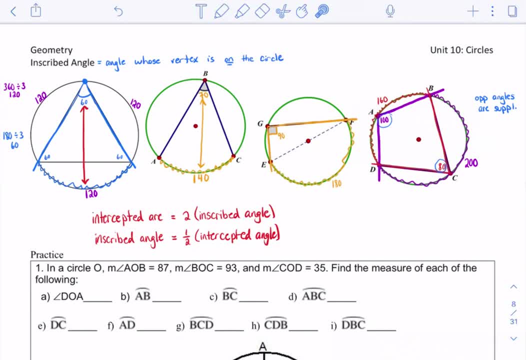 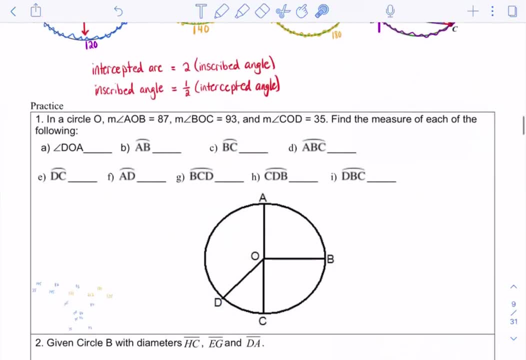 Study those and you should be able to solve then practice one and two. So would you like to go through one of these together? Mrs Telhami, Sure, We're going to skip number one. so if you guys want to try that, that's your practice problem. 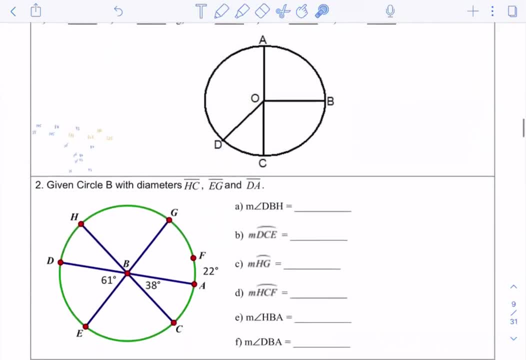 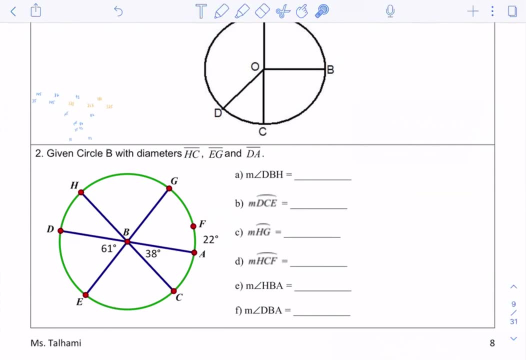 I'll reveal the answers in just a bit. We're going to try number two together. So, Miss Murphy, when you look at number two, what kind of angles do you already see we have here? Well, I see the given angles and I am immediately thinking that opposite angles, vertex angles, exist in this picture. 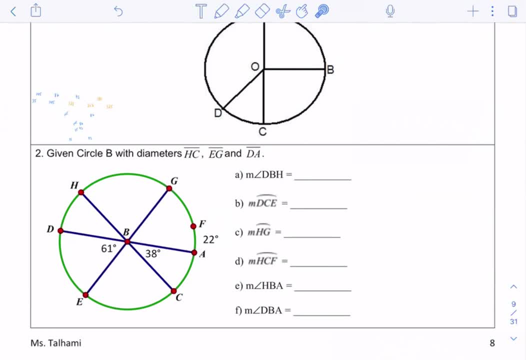 Oh, we do, because we have a bunch of straight lines. And if I also think back to what we just learned- central and inscribed- which angles do I have more of here? or maybe all of Central, because they're all linked to the center of the circle. 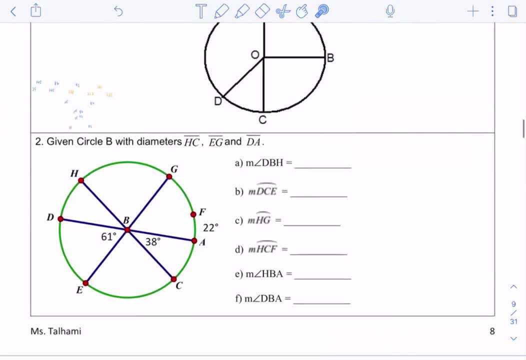 Cool. So central is the same. So I know that this is 61 degrees and this is 38.. It's asking me to find the measure of angle DBH. So DBH is this angle right here? What do you know? That's a vertical angle, so that means it's equal to the opposite of 38.. 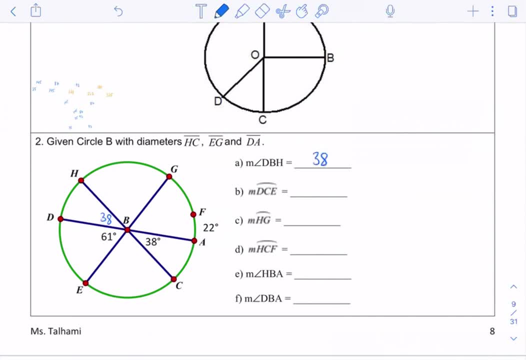 Good, So 38.. So since I know that's a vertical angle, maybe I should do the other vertical angle as well. Yes, So this right here is 61.. Now it says the measure of arc, DCE. So I have to go from D to C to E. 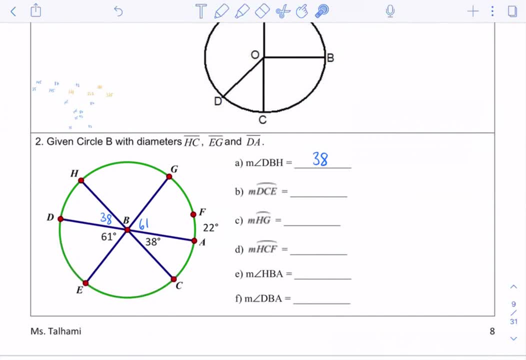 So now some of you might want to go this way, But notice that I'm passing through E, so I can't do that. I have to go from D to C to E, So, if you notice, it's almost the full circle. 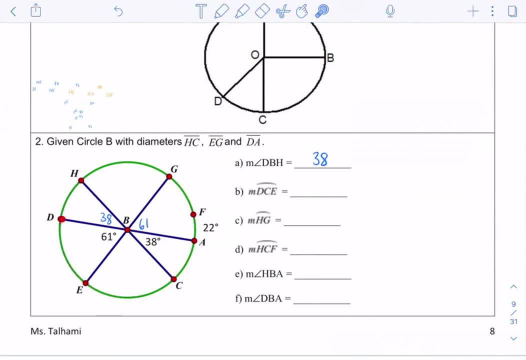 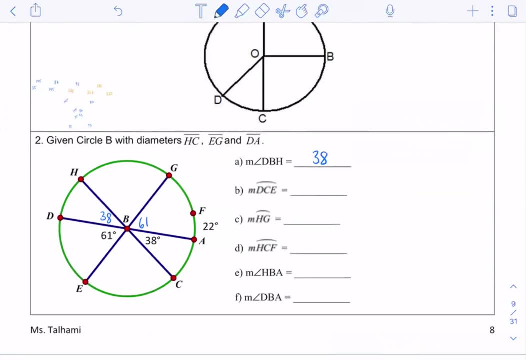 It's everything but this right here. So how many degrees are in this arc? Well, it must be the same, because central is same, So that must be 61.. So everything but the 61 means 360 minus 61. Well, 360 minus 60 is 300, minus one more is 299.. 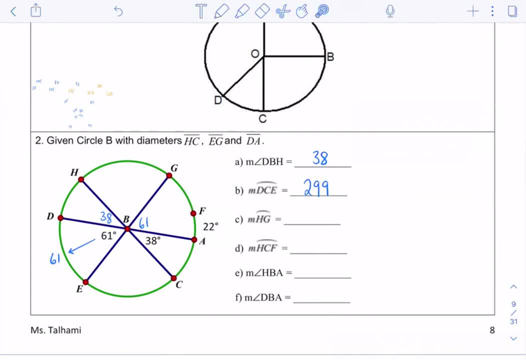 Good, Then we want arc HG. That's this arc right here. Well, this is going to be a little challenging, but here's the thing I do remember, Mrs Tahami always saying that on every line, the sun does shine. 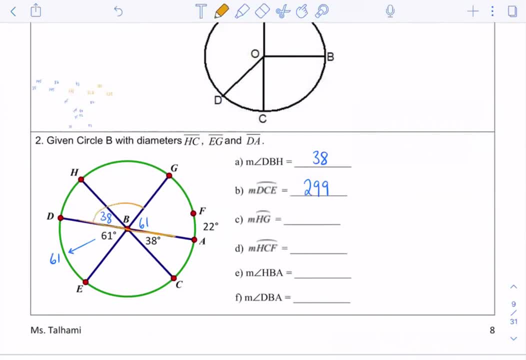 Every line the sun does shine, meaning that all of the angles sharing that line, all those adjacent angles, must add up to 180, because it's a semicircle. So if I do 180 minus the 38, minus the 61,, I get 81.. 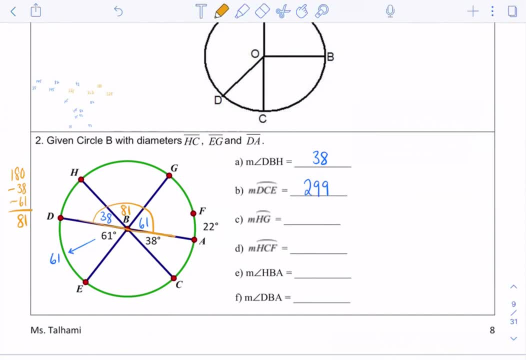 So this is 81. That means this has to be 81. Because central is same Good And might as well label this one 81, since we have it. Then I want arc HCF. So here's H to. oh, I'm passing through F, so I'm going the wrong way. 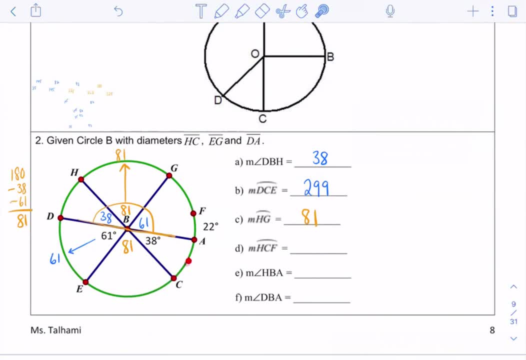 HCF. Ooh, that's interesting. Look what happens here. If this is 22,, do we know how much this one is? Well, altogether, GA is 61.. And if we already have 22,, then 61 minus the 22 would leave me with 39 for GF. 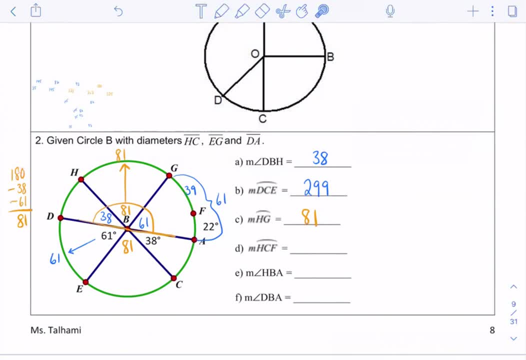 Cool, All right. So that means we want to go from H to C to F. So I mean you can add all these arcs up or you could tell yourself it's almost a full circle. It's everything but the 39 and the 81.. 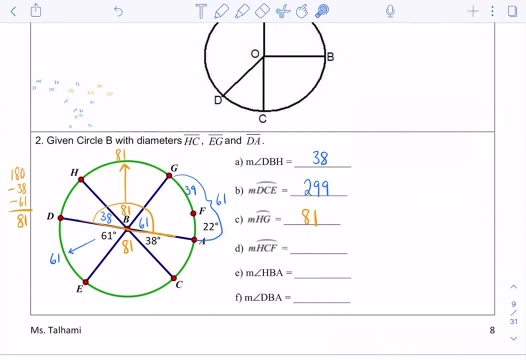 So I can subtract the 39 and the 81.. I can subtract the 39 and the 81 from 360, and that will give me whatever is left here, And that would be 240.. That is a shorter way of looking at it. 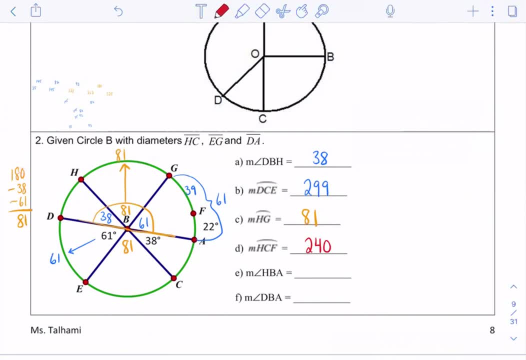 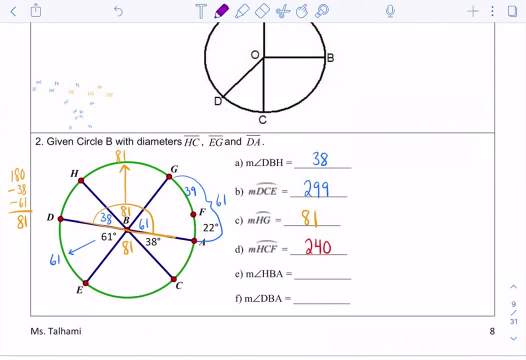 Or you could have, like you said, added up the 38,, 61,, 81,, 38, and 22. And you would also get 240.. And then we have here angle HBA. So that's this angle right here, HBA. 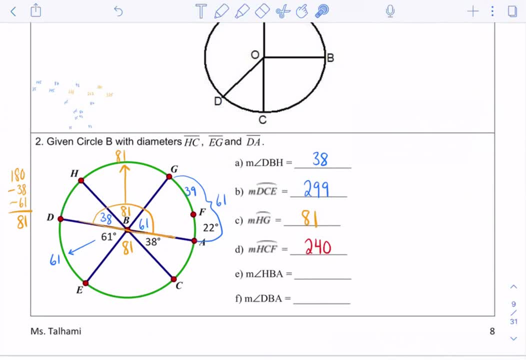 So that's the combination of 81 and 61, which is 142.. And angle DBA. Ooh, what kind of angle is angle DBA? DBA is a straight angle which is a half a circle- 180.. 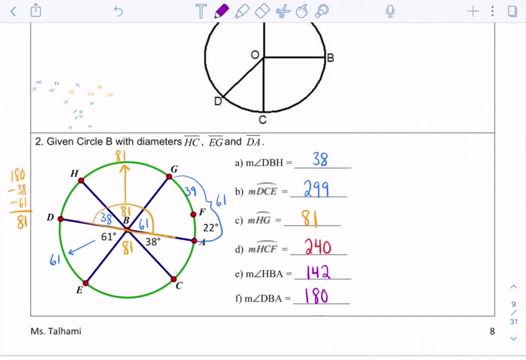 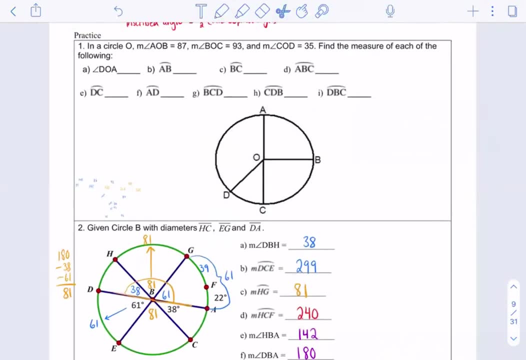 Wonderful. Okay, So from this point on, students can practice some of these ideas, maybe on the next page Right, And they could do number one right now And then, if you want to pause it and try it and come back in just a minute, I'm going to put the answers. 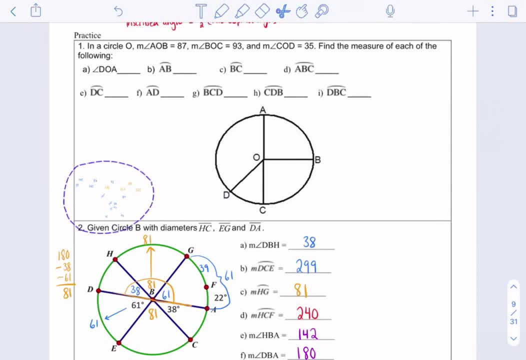 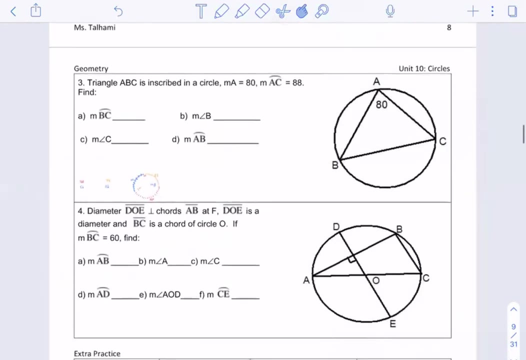 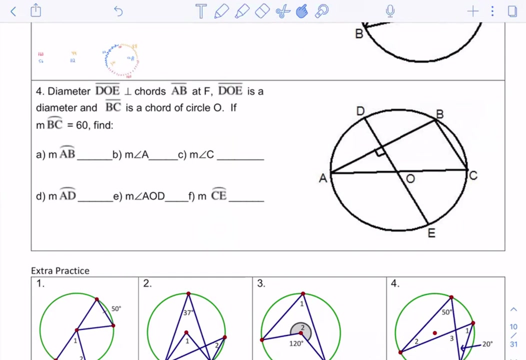 There we go. Excellent, Then on the next page we could try number four with them. Okay, And I'm going to go to my meeting. I'd love to stay. Thanks, Ms Murphy, We'll talk soon. We'll see you on Friday. 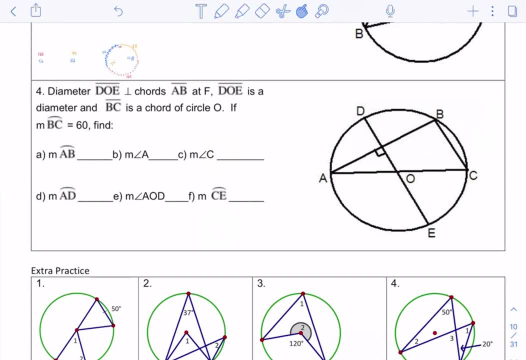 Another A day. Thanks everybody who's been logging in and clicking on those green puzzle pieces and getting your 70% participation credit. Yes, It matters, Thank you. Nice way to earn a great fourth quarter grade. Be well, Bye-bye. 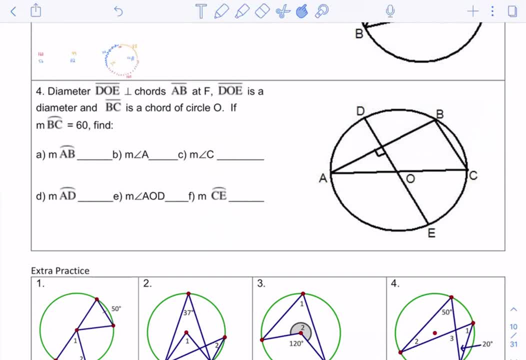 See you later, Ms Murphy. All right, So we just want to finish up here. We want to talk about some inscribed angles. So notice in this picture I actually see inscribed angles right here where the vertex is on the circle. 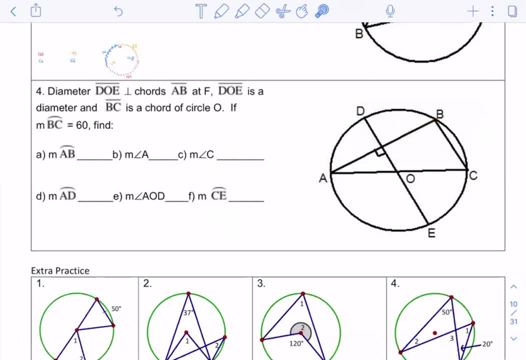 Here's another inscribed angle here and another inscribed angle here. But then I also see some central angles where here is the center of the circle. So here's a few central angles. So it's really important to notice the difference, because central is the same and inscribed is half. 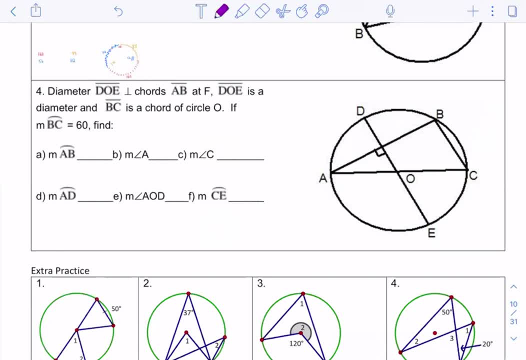 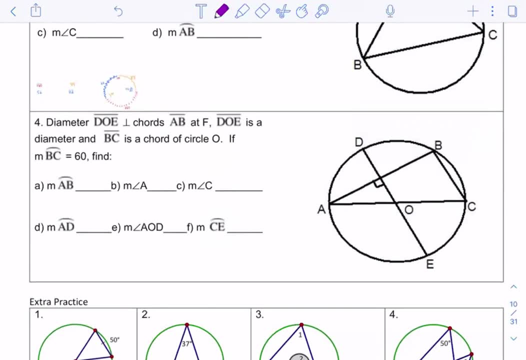 So let's see if we could do this one together. I purposely left the little bit more challenging one to do with you, And then you could do number three on your own. So if you take a look at number four, We have a diameter DOE. 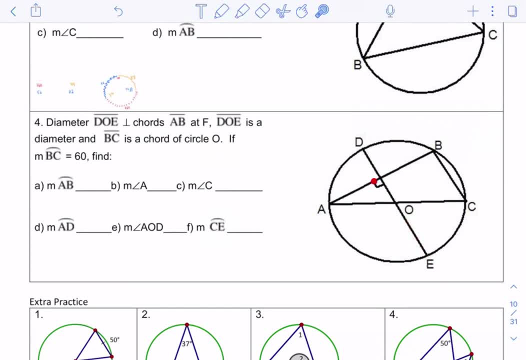 So this is a diameter And it's perpendicular to this chord right here. And it says here that DOE is a diameter and BC is another chord. And then it says: if BC, if arc, BC is 60 degrees, So that's right here. 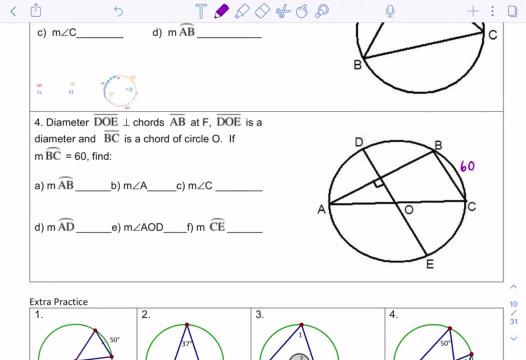 We want to find some other parts of this circle. So the first thing it says is: if this is 60 degrees, what is the measure of arc AB? So the fastest way to get from A to B is this arc right here, Very important for you to notice again the diameters. 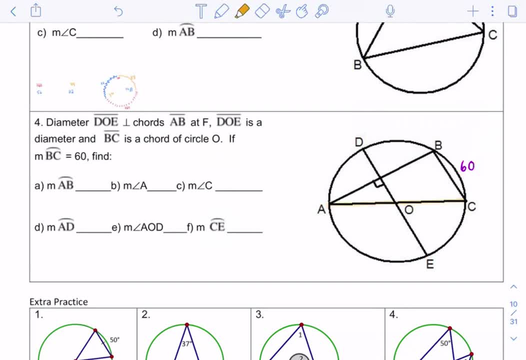 I'm actually going to highlight them because it's really important to see them. They really help us out. So, since AOC is a diameter, that means this must be 180 degrees, And 180 degrees minus this 60 degrees means that arc AB this whole entire thing. 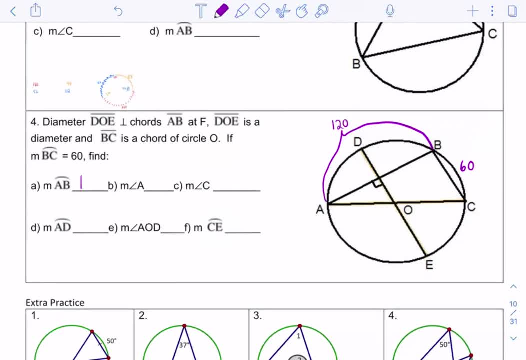 must be 120 degrees. Then it asks us to find the measure of angle A. So here is angle A, right in here. Its vertex is on the circle, So it's inscribed, So it should be half of its intercepted arc. So if I look at what arc it intercepts, 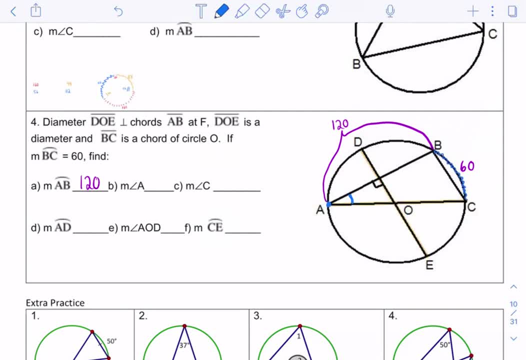 it intercepts arc BC. So it must be half of 60, which means it is 30 degrees. Then I'm asked to find the measure of angle C. So that's this angle right here, If I open up, to see where angle C intercepts. 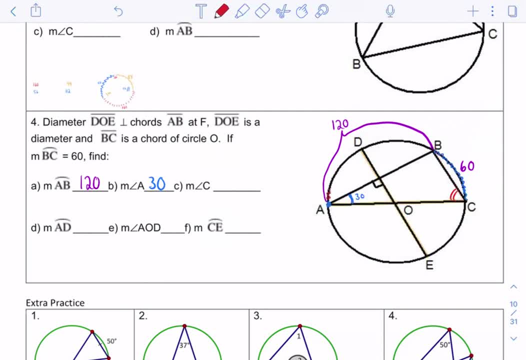 it actually intercepts this arc right here. Now, if that arc is 120 degrees, that means C has to be half because it's an inscribed angle. So that means this is 60 degrees, So that means angle C is 60.. 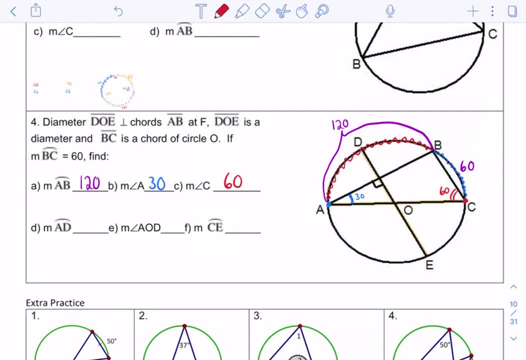 Then it says: find the measure of arc AD. So now this is going to be a little bit of a thought process, because AD, if you look at the arc AD- let me pick a color I haven't used Here- is arc AD right here. 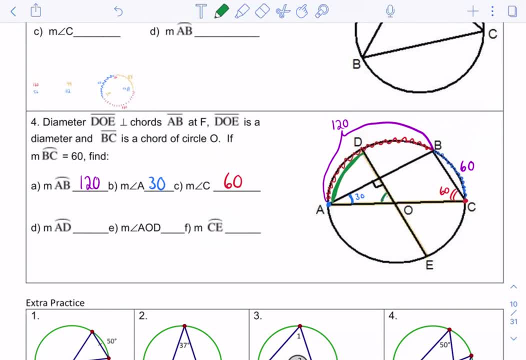 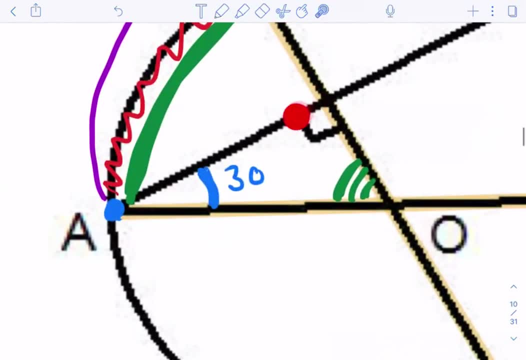 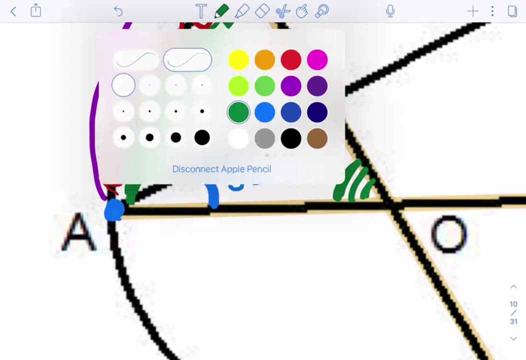 So it should be the same as this central angle right here, which I don't know yet, But if I zoom in, take a look at what you have here. You have a triangle And in that triangle you already know that this is 30.. 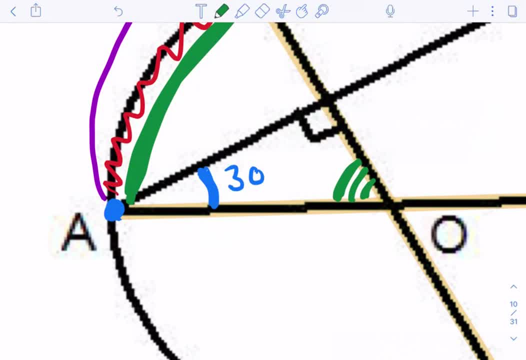 And you know that this is technically 90. So if you know that's 90 right here and this is 30 right here, the angles of a triangle add up to 180.. So 180 minus the 90 minus the 30 means this is 60 degrees, right there. 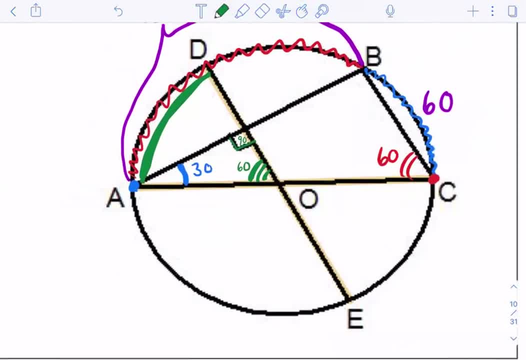 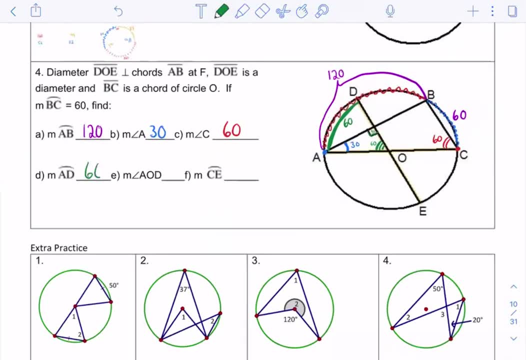 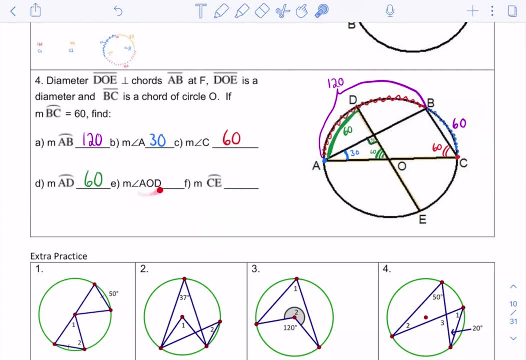 Or it's a 30-60-90, for those of you who remember. So that means arc AD has to be the same as its central angle. So it must mean that arc AD is 60 degrees. Then the measure of angle, AOD. 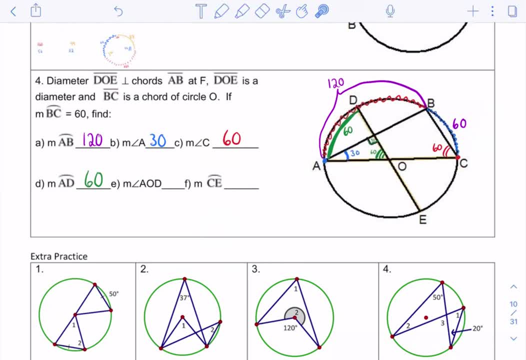 Oh, we just found that That would be 60 degrees. And then it asks us for the measure of arc CE. So CE is right here, So it should be the same as its central angle, which is right here Now, if you notice. 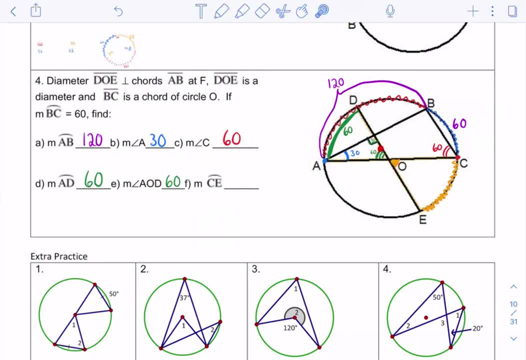 this is a vertical angle to this angle right here, So it's actually also 60 degrees, which means its arc is 60 degrees. I feel like I said 60 degrees too much in this problem, But yeah, so there you have it. 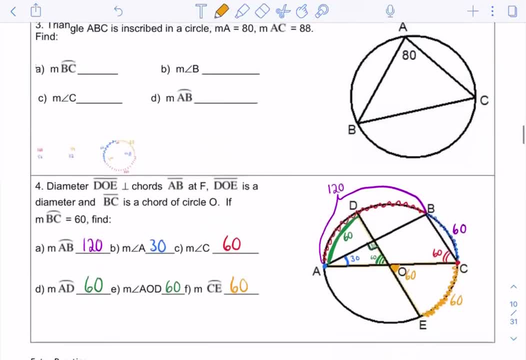 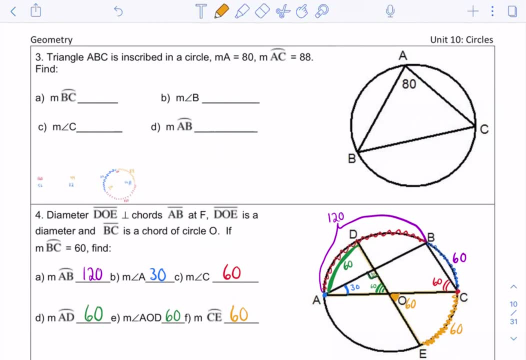 It was a little bit challenging, but doable. So here's an easier problem. Why don't you try number three? Pause it. Come back in just a minute or so. when you're done, I will have the answers up. Okay, so hopefully you completed the problem. 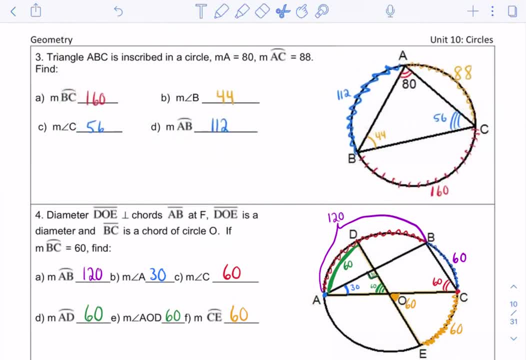 I've had the answers ready for us here. There we go. Oops, just a little angle. So there you have it. It's color coordinated, so if you want to check it, you can check. And then one more set of examples, for you are right here.